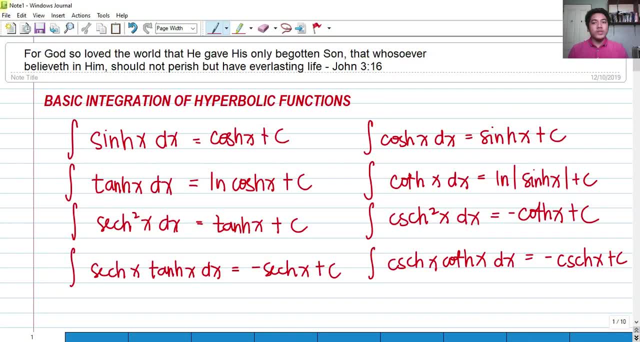 so for today we're going to talk about basic integration of hyperbolic functions and we must at least familiarize ourselves with the formulas involving hyperbolic functions. so we can see, here we have eight formulas in in integration of the basic integration of the hyperbolic functions. so 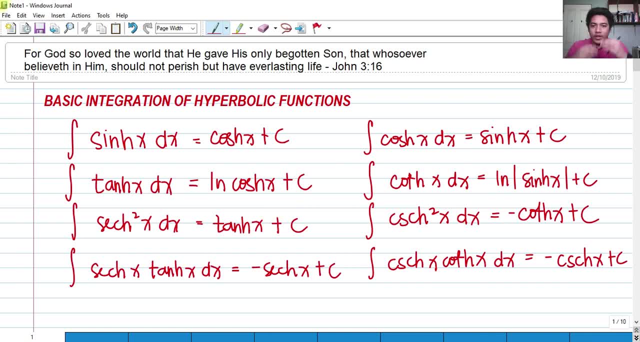 uh, i advise that you take a picture of this or you take down notes in this formulas, as we are going to solve some problems, okay, and in integrals we have so many formulas. that's why there is a different formula. for the integration of trigonometric function, there is a different. 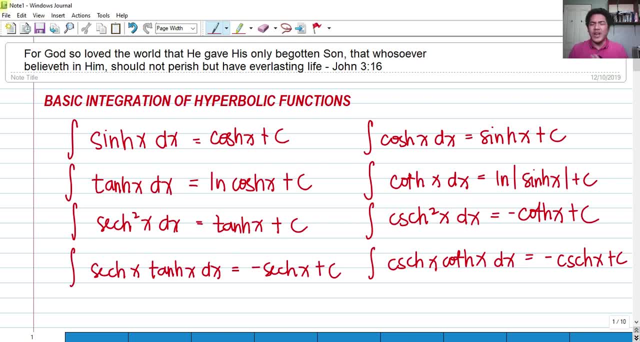 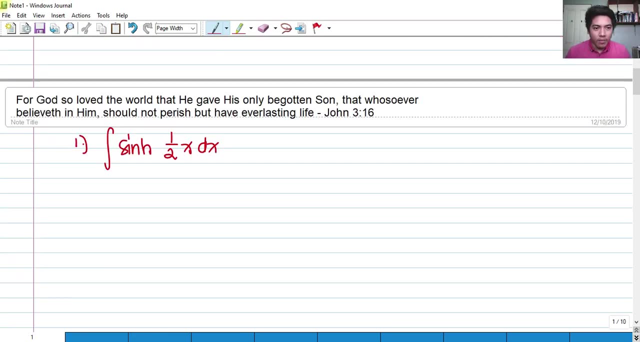 formula in hyperbolic function and so on and so forth. we have so many formulas here in integrate in integral calculus, so might as well you take note of these formulas, okay, so let's get started. okay, so let's start by integrating this problem, so the integral of hyperbolic sine. 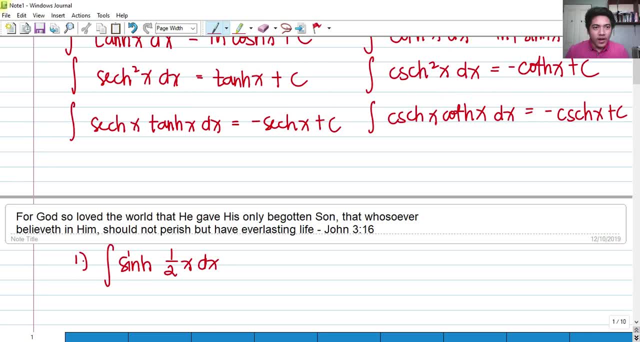 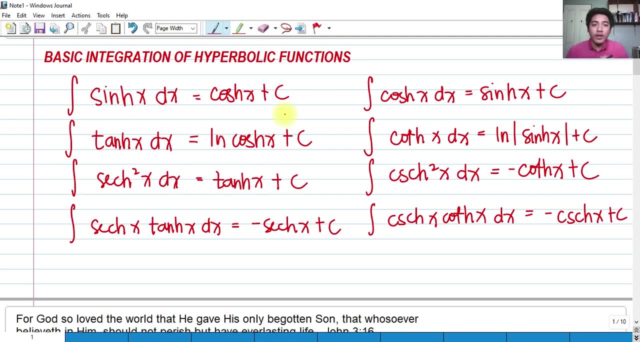 x, dx is equal to the hyperbolic cosine of x plus c. okay, there is no negative, whereas in trigonometric function there should be a negative, but in hyperbolic function there is no negative here. so what we can see here is we cannot directly integrate this as hyperbolic cosine of one half x. 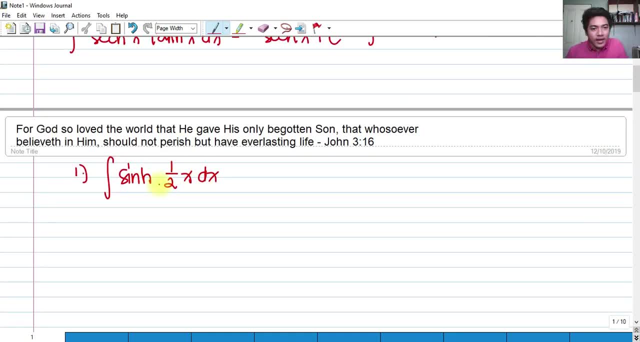 plus c. why? because our formula only tells us that the integral of hyperbolic sine x- dx is equal to the integral of hyperbolic cosine of x plus c. okay, so we can see that the integral of hyperbolic sine x- dx is equal to the integral of hyperbolic sine of x plus c. okay, so what we have to leave? 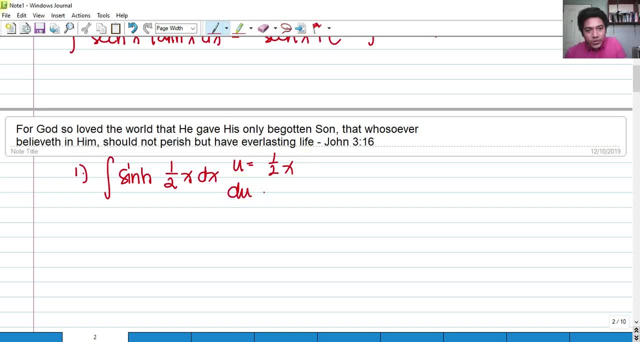 u as one half of x- okay, and du as one half dx- okay. so in other words, we will be using the u substitution here. okay, so we have the du is one half dx. this does not have a one half, okay, so we're going to have a correction factor of one half and, of course, the reciprocal of this correction. 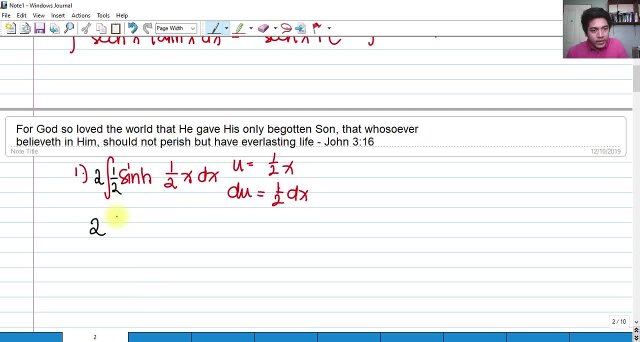 factor outside of the integral sign. so we have two integral of a sine, hyperbolic sine of let u, one half x, and then we have one half dx that is equivalent to u. now, we can now integrate this function. this is also the same as sine of x or hyperbolic sine of x, okay, whereas our 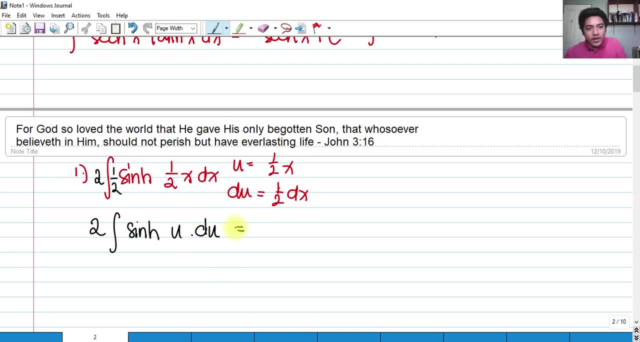 variable. only here is u. okay, so if we integrate that, that is two hyperbolic cosine of one half x plus c, okay, you, our u is actually we replace it already by one half x, because originally our variable is in terms of x. so that is our answer. so for number, 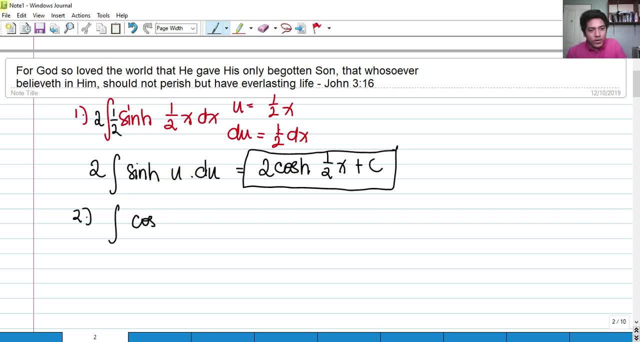 two. okay, we have a hyperbolic cosine of 2x, dx. okay, in this case, we will be also adding a correction factor of two inside of the integral, because it will let you as 2x. the derivative of 2x is 2dx, so 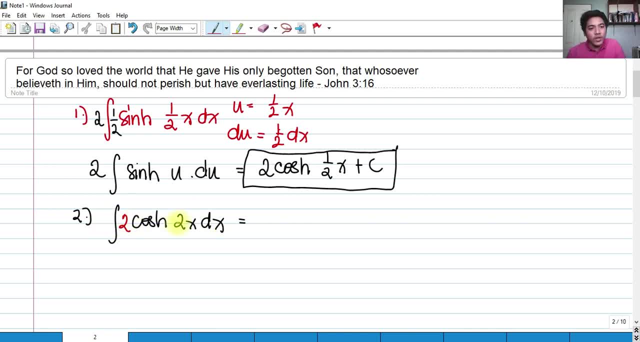 we have to have 2dx here and of course, if we multiply 2 inside of the integral, outside of the integral we must multiply one half here. so our answer here: if we're going to rewrite this by performing u substitution, one half the integral of the hyperbolic cosine of u. 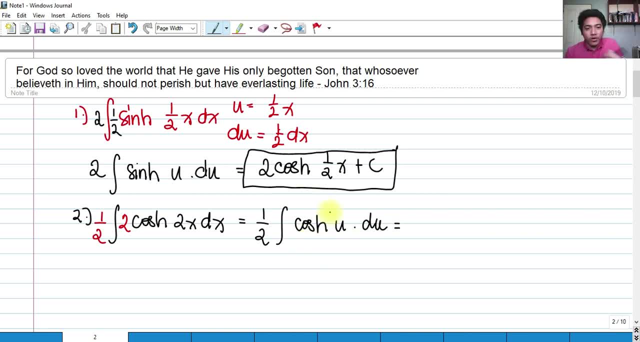 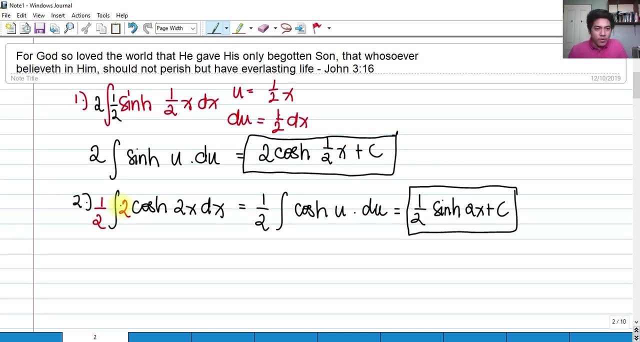 hyperbolic of cosine. okay, the integral of hyperbolic cosine is hyperbolic sine 2x plus c. okay, so that's very simple. okay, for number three, we need to find the integral of hyperbolic second squared of 2x minus one. okay, dx. 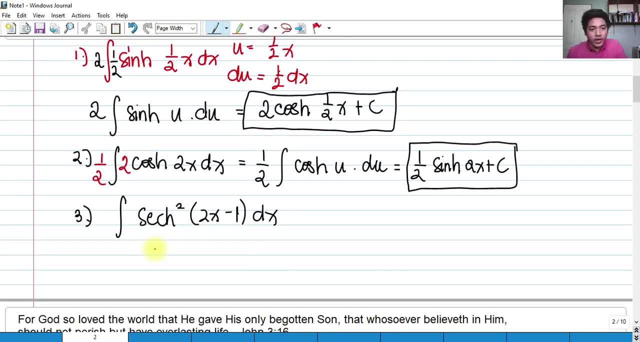 okay, we will be also using u substitution here, in that we make- we have to make u as 2x minus one. the du is 2dx, so that we're we will be getting a correction factor. we will be putting a correction again of two and one half on the outside of the integral. so what will happen here is that we will. 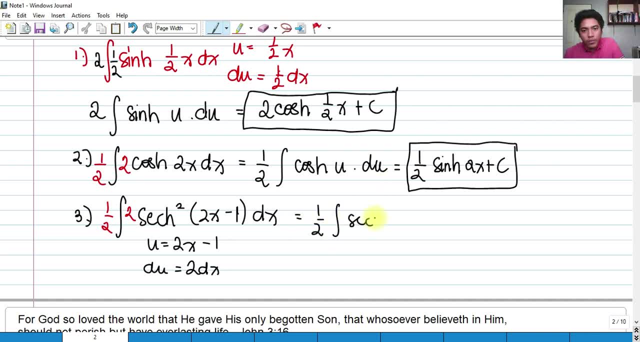 be having one half integral of hyperbolic second squared. u multiplied by the integral of cuando c s into the integral of half is equal to c square. so that is the upper half integral of hyperbolic sec second squared. Let's look at the second part of this Dak: derivative value of 2x. when we difference. 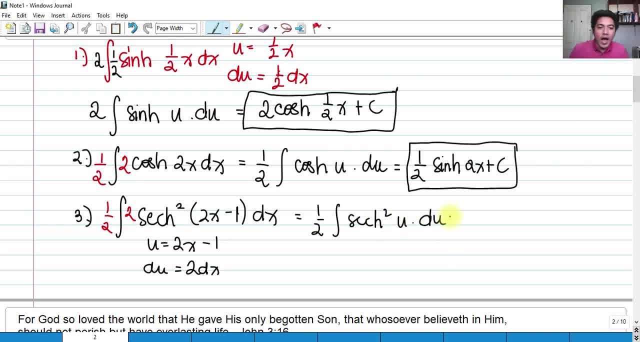 it nosotros integram, And our formula for this is simply hyperbolic. The integral of hyperbolic second squared u, du, is equivalent to hyperbolic tangent. So we have one half hyperbolic tangent of 2x minus 1 plus c. 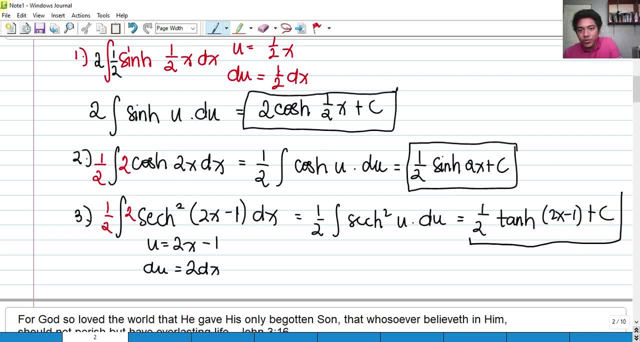 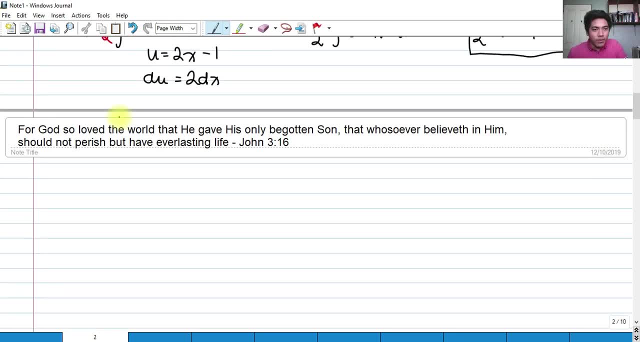 I have already substituted the value of u, which is 2x minus 1, for our final answer. Let's go now to number 4.. It's pretty easy, right, Because this is a basic video, all about integrating hyperbolic functions. 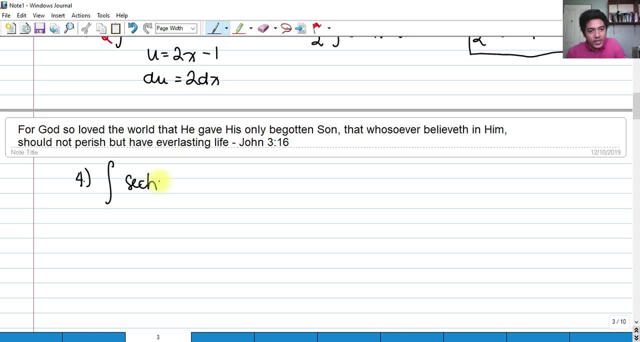 So we have the integral of hyperbolic second x- dx. This is a tricky one. If we rewrite this hyperbolic second, we have 1 over hyperbolic cosine of x- dx. That's an identity in hyperbolic. So what will happen here is if I'm going to add a hyperbolic cosine of x in the numerator, 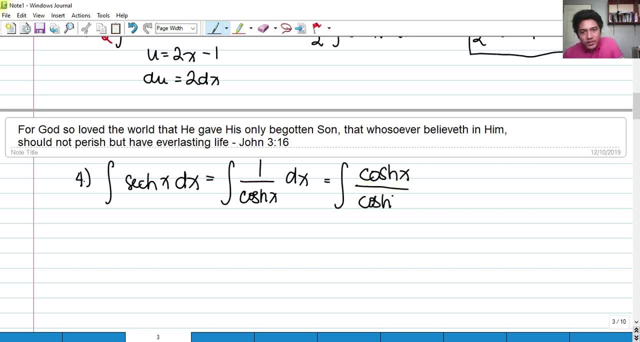 over hyperbolic cosine squared, x, dx. here this integral is equal to this, because hyperbolic cosine of x divided by hyperbolic cosine of x squared is still 1 over hyperbolic cosine of x, And we must take note that there is an important identity involving hyperbolic function. 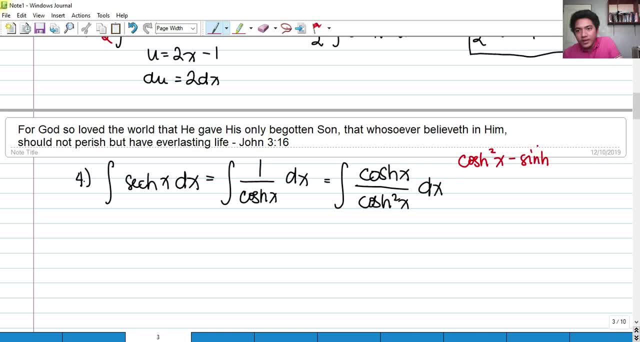 wherein we have this identity, wherein we have hyperbolic cosine of x squared minus hyperbolic sine of x squared, is equal to 1.. So if I'm going to replace hyperbolic cosine of x squared, what will happen is that I will be having hyperbolic cosine of x over 1 plus hyperbolic sine squared of x here dx. 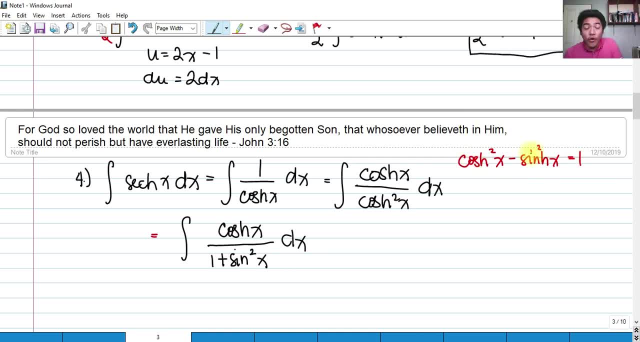 because of this relationship or identity. So if I'm going to transpose this on the other side, I'll be getting this formula, okay. So, and again, we can what? This is a little bit tricky because if we have this, 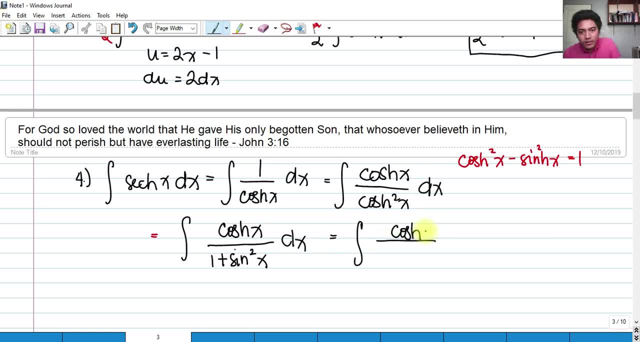 if we write this integral in the form of this: okay, 1 squared plus hyperbolic sine squared. okay, This is hyperbolic sine squared. I'm so sorry, This is hyperbolic. okay. So for the function of x: okay, we can see here. we have a dx here. 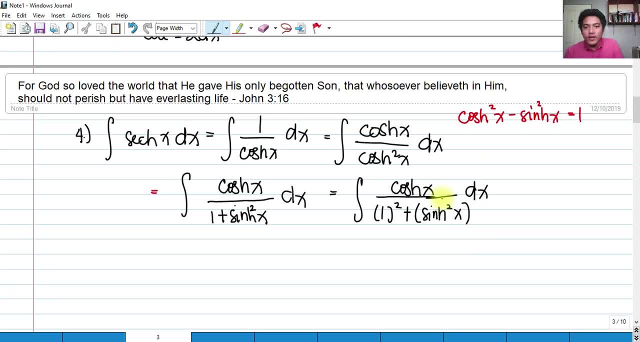 We can see here that this is an integral yielding to an inverse trigonometric function. So it is in the form of: let's say we have. it is in the form of dx over 1 plus okay, u squared, or this is a squared, okay. 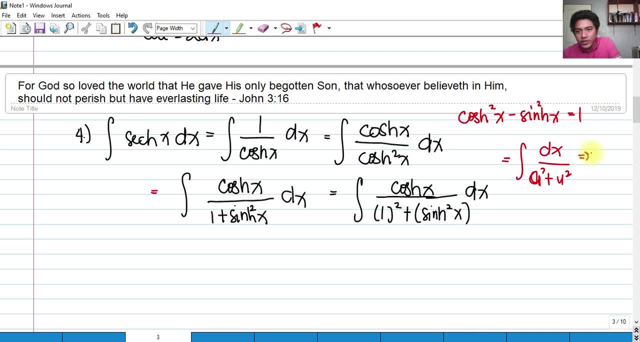 And this integral is actually yielding to an inverse 1 over a. okay, let me just rewrite this so so for you to get it. so what i'm trying to say is: we have, if we have, an integral of dx over a squared plus u squared, okay, that is an integral yielding to. 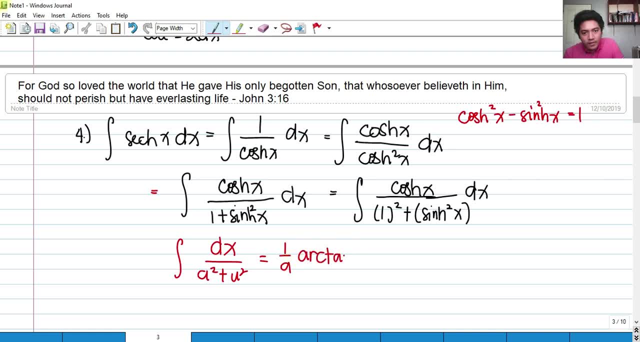 arc tan 1 over a arc tan of x over a plus c, which is we're going to analyze. this is our a, okay, and this is our u. i'm sorry, this should not have a squared here, but rather we have a hyperbolic sine squared here. we factor out the square sine, okay, but this is still equal to this. 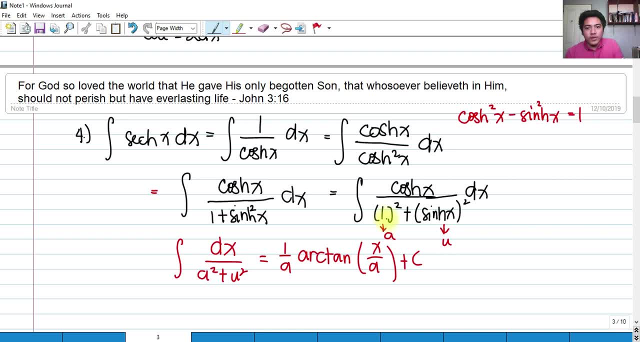 so this is our u, this is our a. so if we're going to put it into this form, okay, if we're going to let u here as hyperbolic sine of x going to get a hyperbolic sine of x, going to get a hyperbolic sine of x. 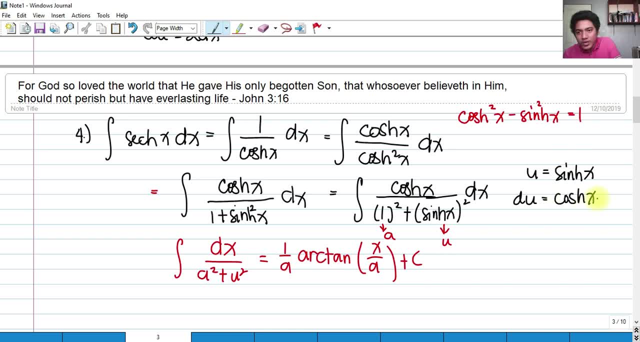 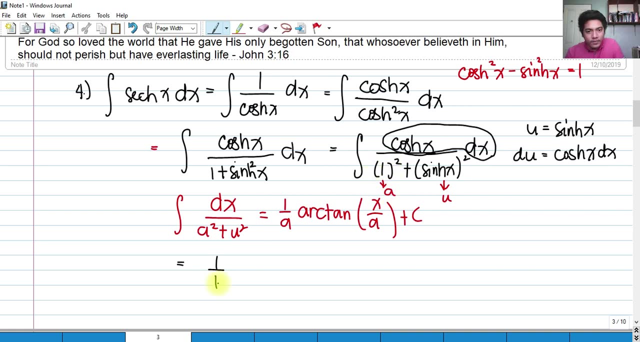 derivative of hyperbolic sine, that is, hyperbolic cosine of x, dx, which is available here in our numerator. we can perform therefore this: so what will happen is that we have 1 over our a. is 1 arc tan of x? what is our x? okay, or i mean, this would be, this would be. 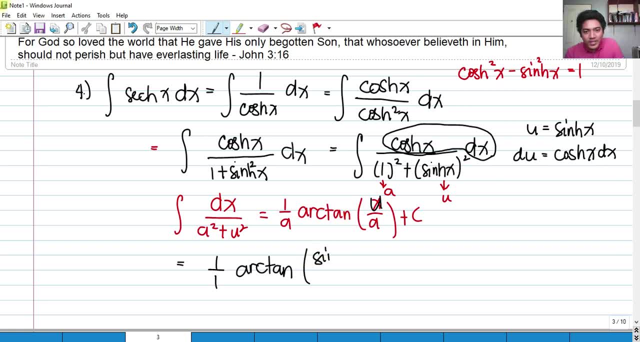 this would be u okay, so hyperbolic sine of x over a, which is 1 plus c drink, and if we're going we're going to simplify this, we'll be having our done off the hyperbolic sine of x plus c. so this should be our uh answer. 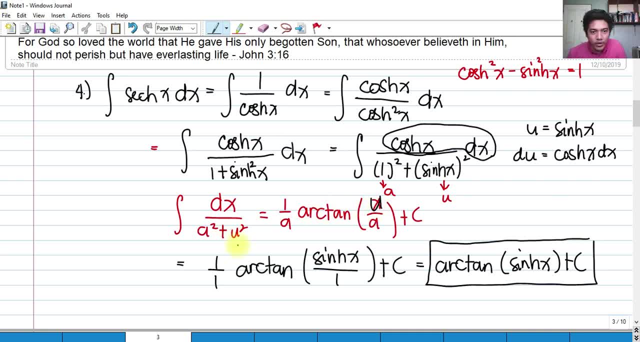 to our problem. so i my mistake. this should be u. if i'm going to use u, doesn't matter. if you use x here, then definitely this would be the same 속 for problem. but i'm gonna exemplify these two. so if you're gonna keep these two as my sus package, 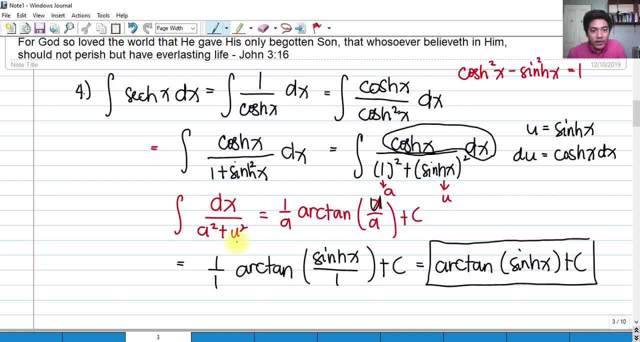 the answer would be u, donc eu can't be can to have u, then it doesn't matter. if you use x here, then it won't refer to his. an two fibra would be x, okay, but in our formula i used u so that this would be also u and not x okay. 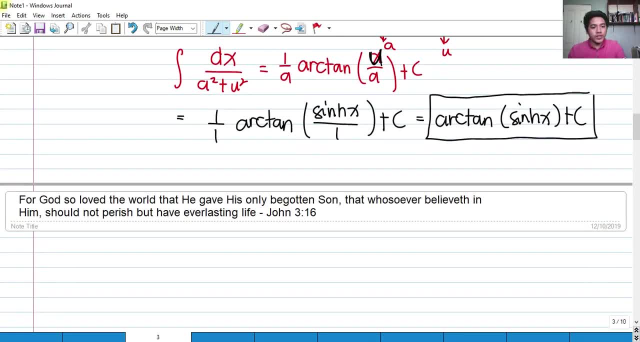 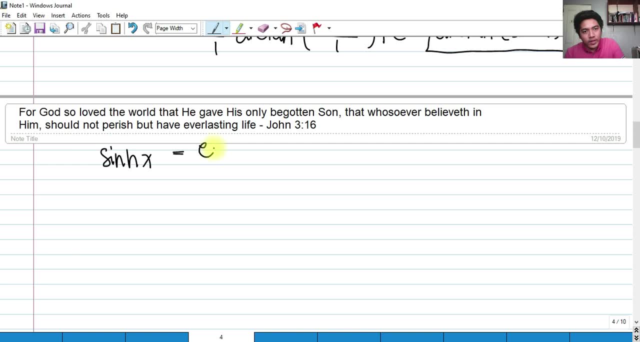 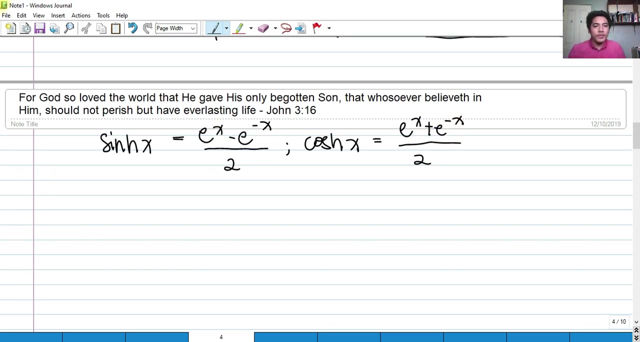 okay, let's proceed, but before proceeding, it's also important to take note that hyperbolic sine of x is equal to the following: e raised to x minus e raised to negative x over 2, and we have the hyperbolic cosine of x. is e raised to x plus e raised to negative x over 2. okay, so we need this. 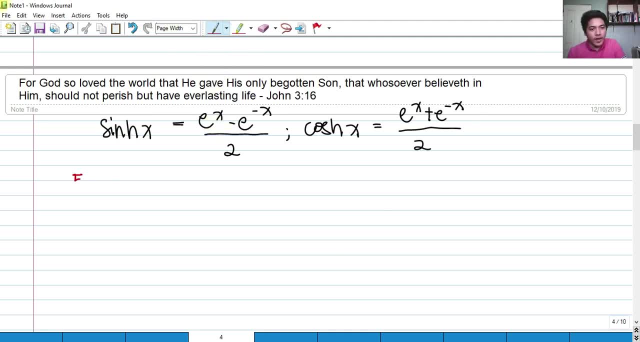 for our fifth example. so we have number five: the integral of e raised to x, hyperbolic cosine of x, dx. so if you learned already integration by parts, you can perform integration by parts. but what? what i would like to share with you here in our video is that 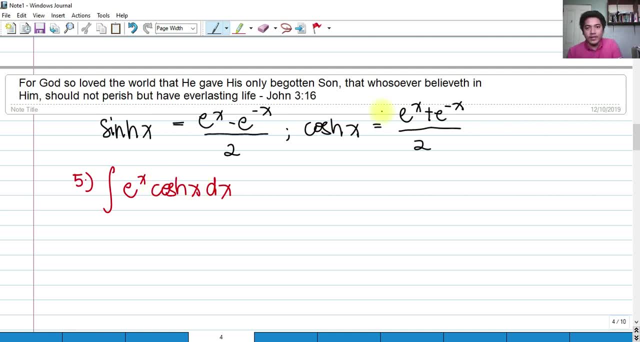 we're going to do is we're going to use the integral of e raised to x, hyperbolic cosine of x- we're going to replace hyperbolic cosine of x by this, okay, and evaluate the integral. so what will happen? we have integral of e raised to x multiplied by e raised to x plus e raised to. 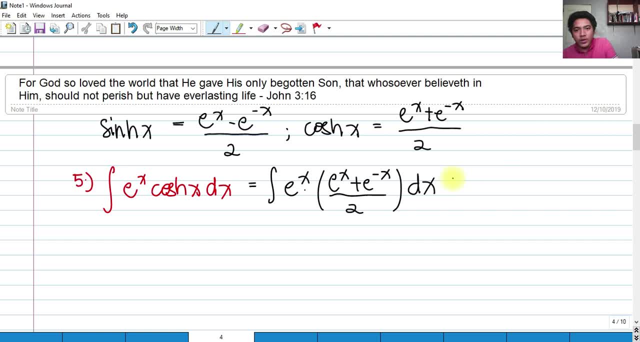 negative x over 2 dx. so if i'm going to multiply this, what will happen? we have e raised to x multiplied by e raised to x- okay, over 2 dx- plus integral of e raised to x multiplied by e raised to negative x over 2 dx. i've already used the property of integral, wherein. 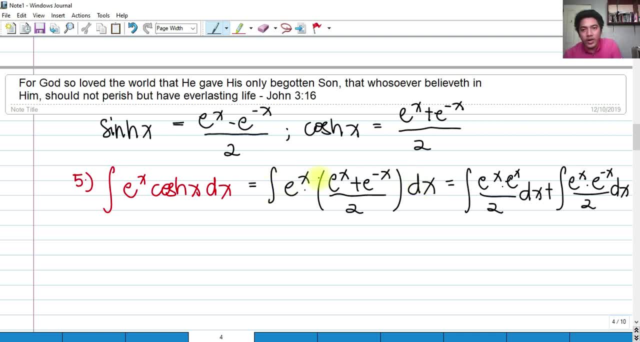 we can distribute dx and as well as the integral sign. so by loss of exponent, this two would become: e raised to 2x over 2 integral dx plus e raised to x, so e raised to x multiplied by e raised to negative x, so their exponents would: 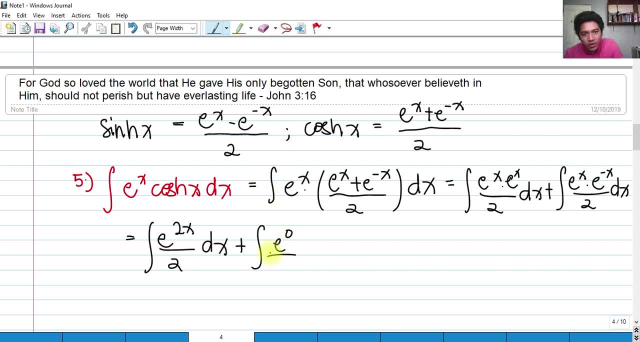 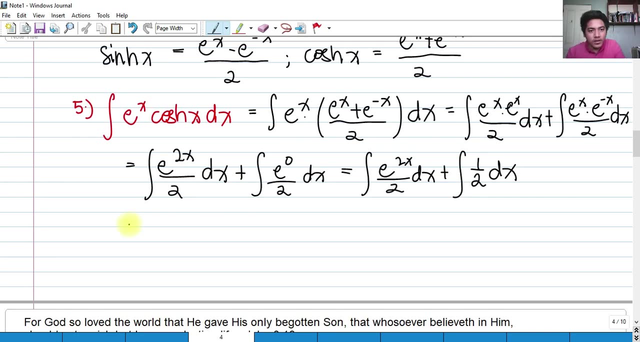 drop and x minus x is e raised to 0 over 2 dx. so we are left with e raised to 2x over 2 dx, plus any number raised to 0 is 1 half dx, so that we can now integrate this. so we have one half. 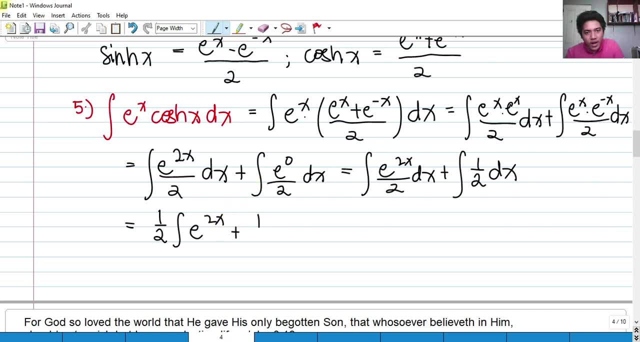 e raised to 2x plus one half integral of dx. i put the constant outside of the integral sign, so we have the integral of this should be one half multiplied by one half. you see, you will have to use u substitution here and if you get a derivative of 2x, that is 2 dx. okay, forgot the. 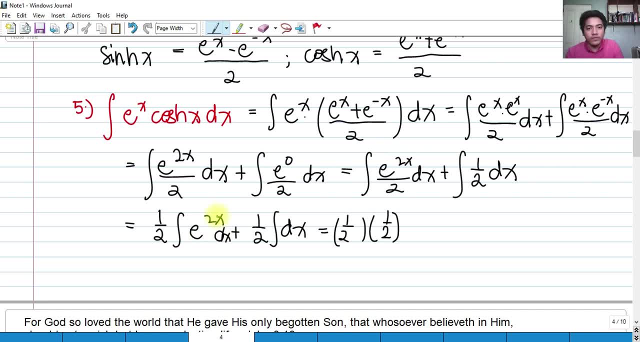 dx here, so 2 dx. then you have to have a correction factor of one half outside of the integral, because derivative of this is 2, so one half times one half. okay, copy the same. okay, e raised to 2x. oops, so we have e raised to 2x, then plus 1 half. integral of dx is x plus c, so we have. 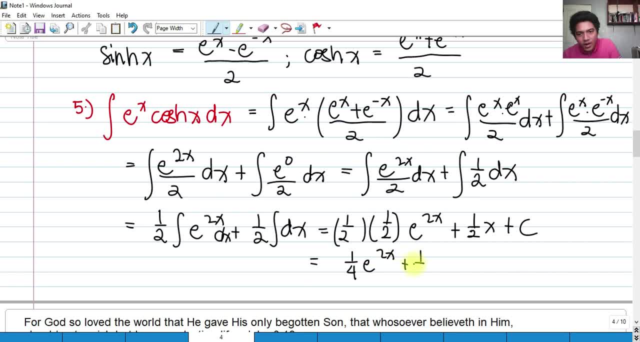 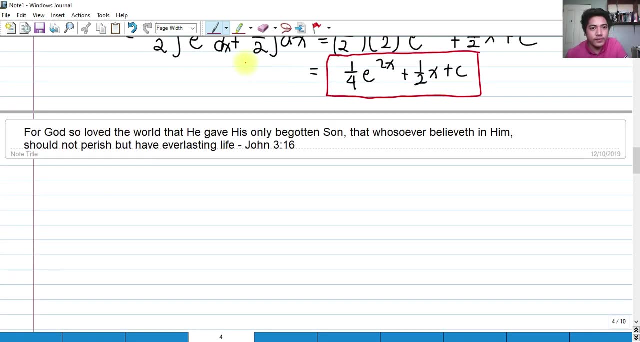 now 1 fourth e, raised to 2x plus 1, half x plus c, and we have now our answer for this problem. so for our next problem we'll be having this problem. so we have number six, the integral of x hyperbolic sine of x, dx. okay, so we'll be using again the substitution of 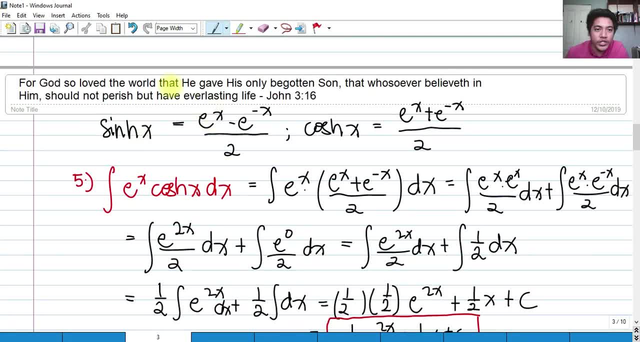 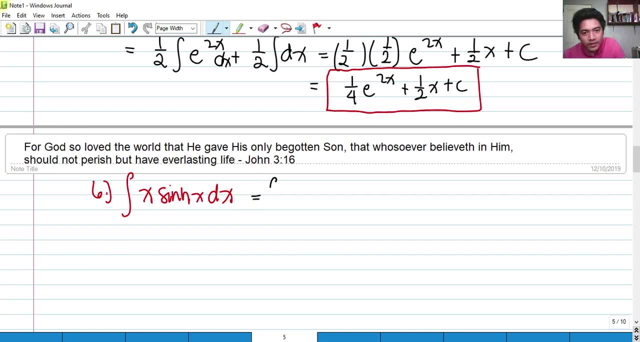 hyperbolic sine of x, the definition of hyperbolic sine of x, which is this: e raised to x minus e raised to negative x over 2. so we substitute that we have integral of x multiplied by e raised to x minus e raised to negative. 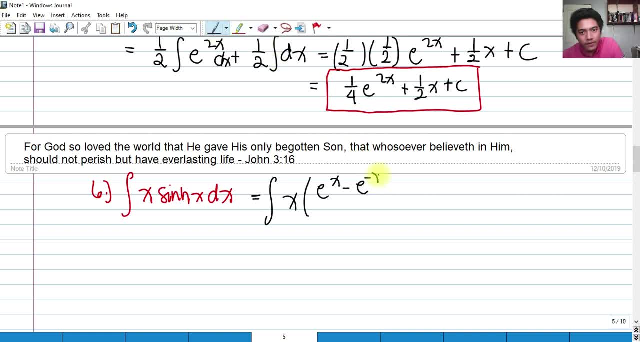 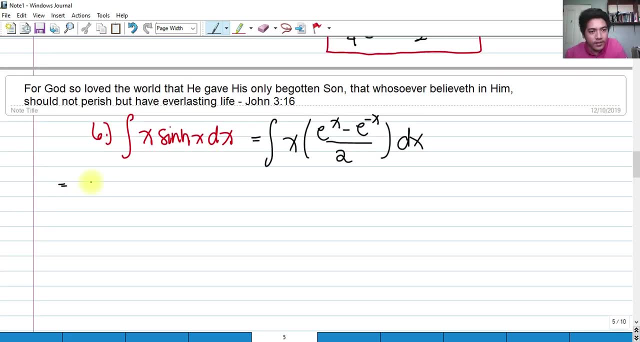 we have x over 2 and dx. so if i'm going to distribute the x in our function here, so we have x e raised to x minus x, x e raised to negative, x over 2, dx. okay, i can separate those two where you and i will be. 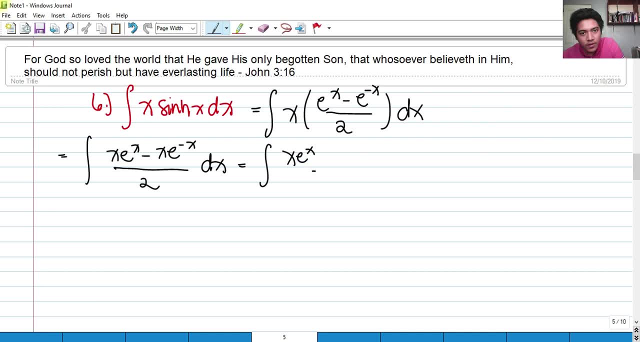 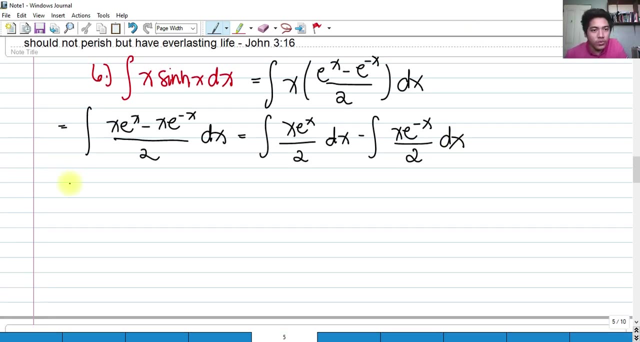 having x integral of x e raised to x over 2 minus dx, minus the integral of x e raised to negative x over 2 and dx. okay, so what will i do to simplify the integral is i have to, uh, let the one half outside of the integral sign. okay. 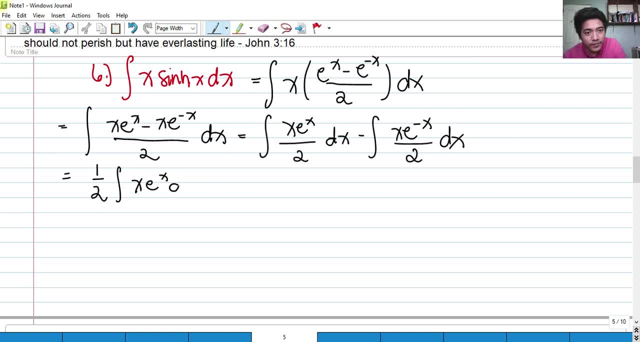 so that i have x? e raised to negative x dx, minus one half the integral of x. x e raised to negative x dx. okay, and i can perform integration by parts here. i'm going to let u as x, my du would be dx. okay, and my dv here would be e raised to x- dx and our v is simply e raised to x. the same here. 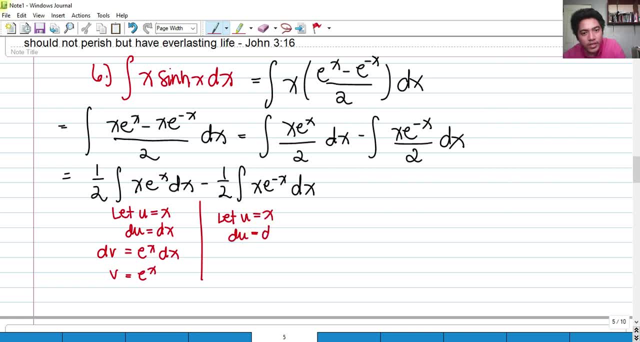 let u as x, our d would be dx and my dv would be e raised to negative x, dx and my v. if i'm going to integrate this, i would be having a negative, because this is a negative e raised to negative x. so e negative, e raised to negative x. okay, that. 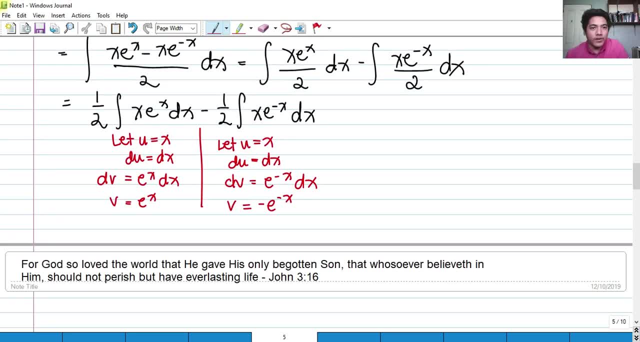 would be my uh parameters. okay, so what will happen here again? we're going to it: perform integration by parts. okay, if i'm going to perform integration by parts, recall that the formula is uv minus the integral of vdu, so i have one half. okay, uv for the first. i. 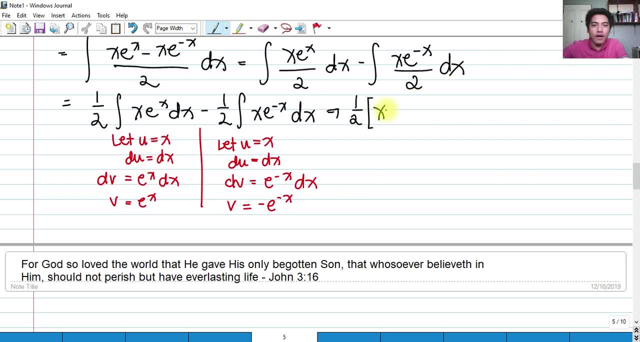 have u x. okay, i have the x multiplied by v e raised to x, minus the integral of v e raised to x. my du is dx, okay, minus one half. okay, v x multiplied by negative x e raised to negative x because here is our u and our v is negative. so 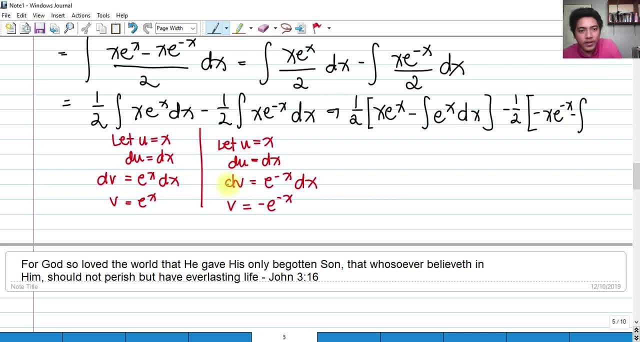 that we have this product minus the integral of v du. our v du is negative, e raised to negative x and my du is equal to dx, simply okay. so what will happen is that one half okay, x, e raised to x. if i'm going to integrate this, what will happen? i'll be having one half also, e raised to x here. 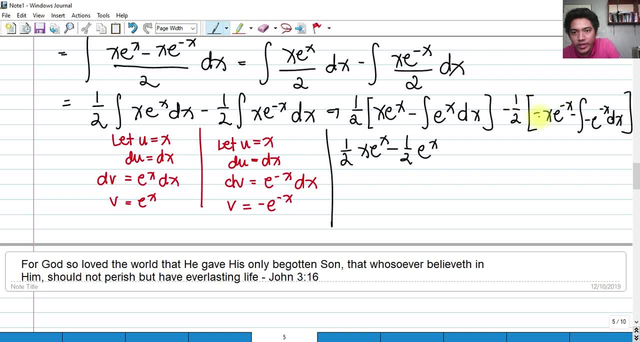 okay, if i'm going to distribute this, we'll be having plus one half x, e raised to negative x and we have, if i'm going to factor out negative here, negative times. negative because this is a minus sign. that would be positive, okay, and multiplied by negative, so i'll be having 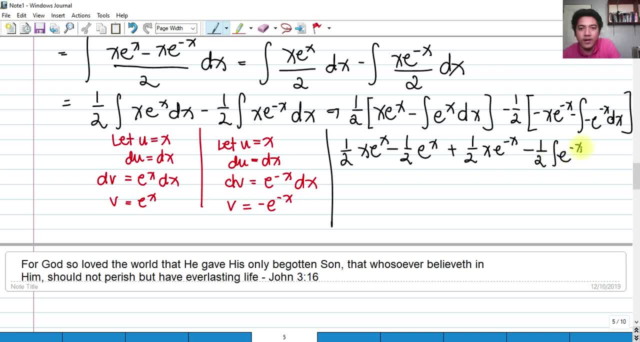 negative. one half integral of v du e raised to negative x. okay, so one half of x e raised to x minus, one half e raised to x plus. one half x e raised to negative x minus. okay, if i'm going to integrate this, okay, if i'm going 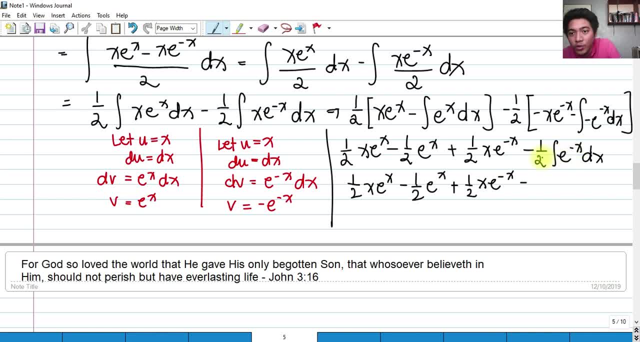 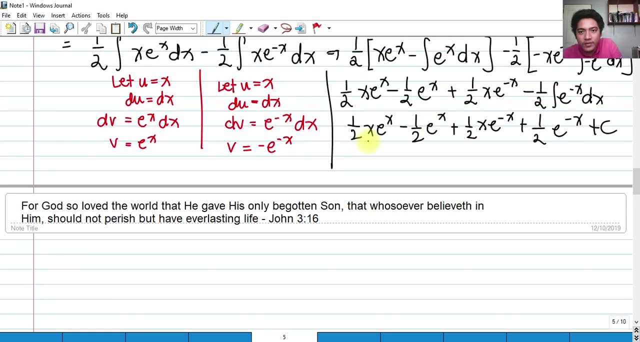 to integrate this. it would produce a negative e raised to negative x multiplied by a negative, that would be positive one half e raised to negative x. okay, so what will happen here? if i'm going- well, of course we have the plus c, okay, if i'm going to rearrange this, okay, such that i'll be picking one half x. e raised to x. 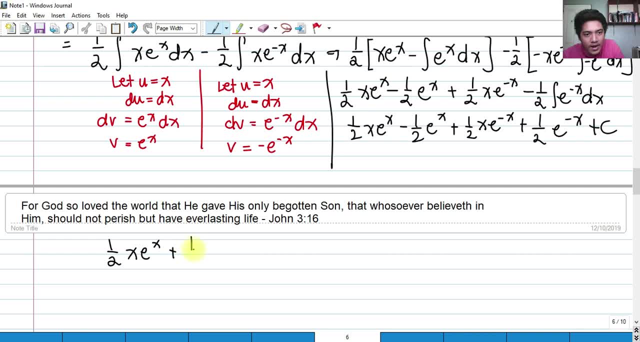 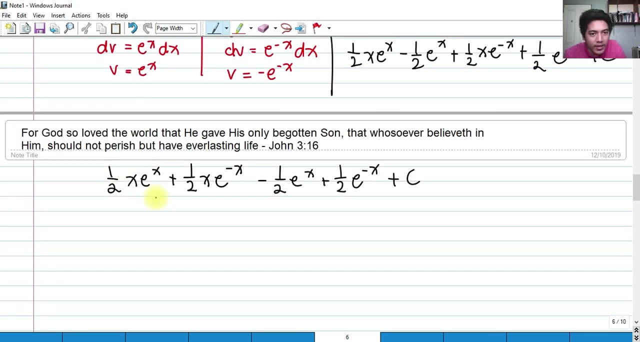 and i have here another one: plus one half x e raised to negative x and minus one half e raised to x. this is that term plus one half e raised to negative x plus c. and if i'm going to factor out x in this term, okay, x in these terms, i'll be having 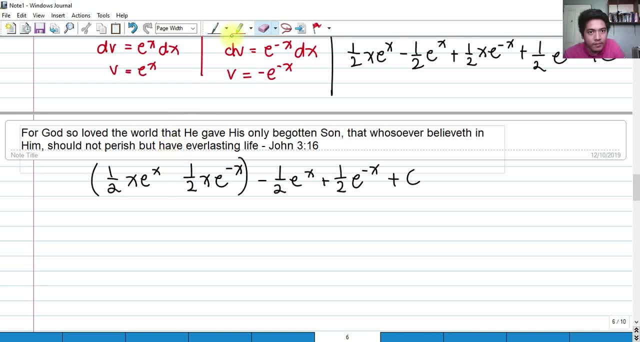 i'll be having this: okay, x would now be x or, sorry, e raised to x. so e raised to x- okay, plus. e raised to negative. x over two, okay, minus. if i'm going to factor out the negative here, we would be having what we would be having: e raised to x minus one half. e raised to x minus one half. e raised to x minus one half. e raised to x. 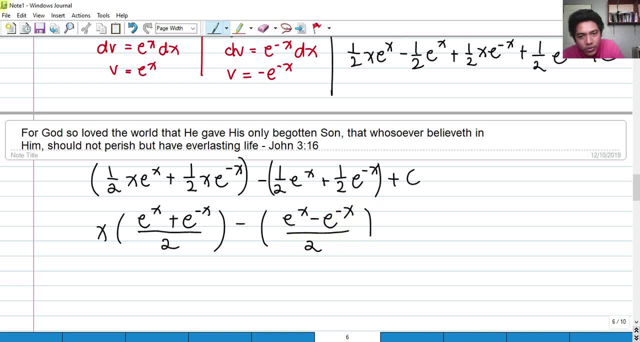 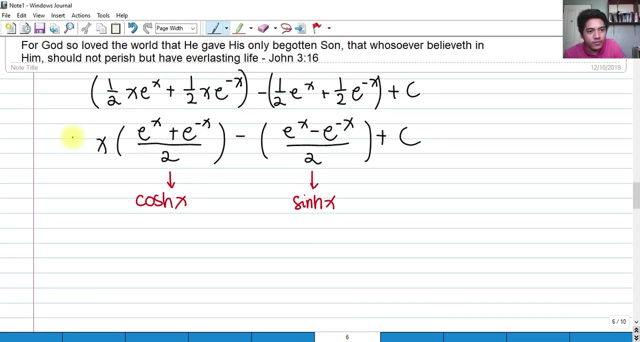 minus e, raised to negative x over two plus c, and if we are going to recall this whole term, this whole term is equal to hyperbolic cosine of x and this whole term is equal to hyperbolic sine of x by definition. so the answer would be: the answer would be x, hyperbolic cosine of x minus right, minus. 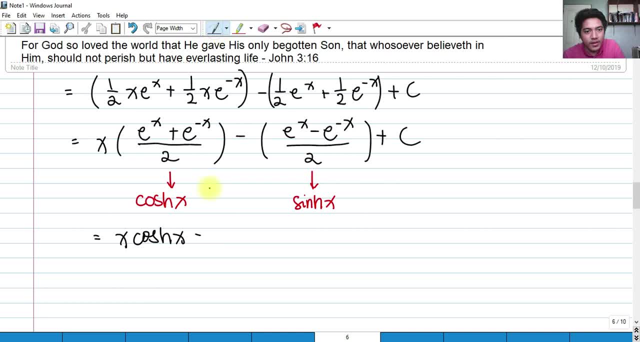 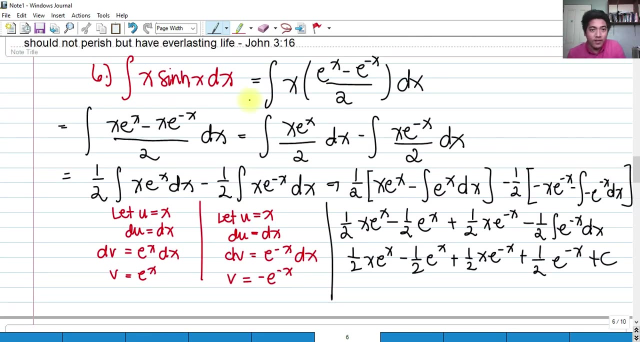 hyperbolic sine of x, hyperbolic sine of x plus c. so that is the integral. that is our answer for that integral, and if you're going to do integration by parts from the beginning here, okay, you'll be arriving at this answer. i've just shown you that this. 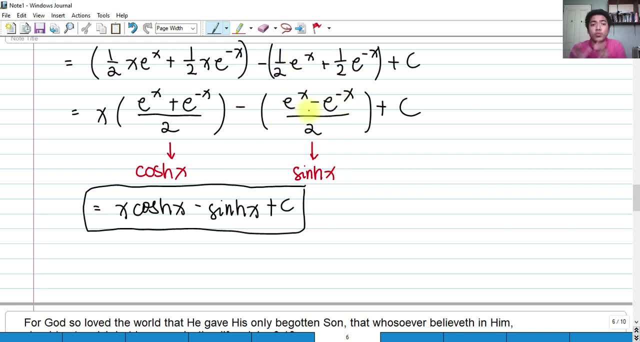 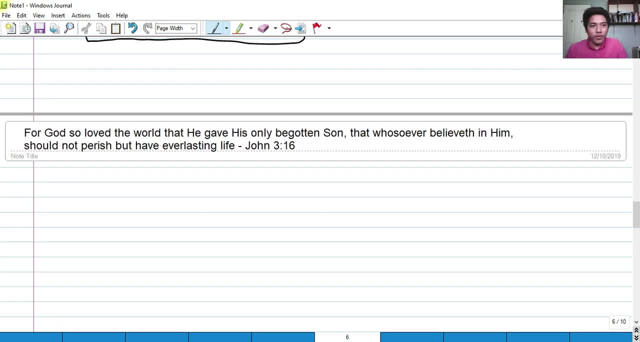 function can be used also if we are going to integrate, and it would yield to the same answer. okay, down to our last example for this video. so we have number seven, if i'm not mistaken. we need to find the integral of the x squared multiplied by the hyperbolic sine of x. 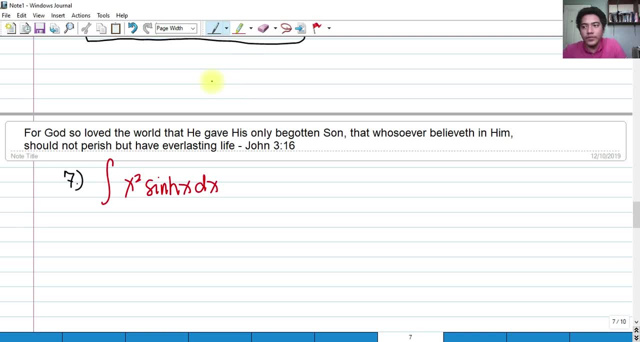 dx. okay. so let's try to use- okay, let's try to use- integration by parts here, okay. so if we're going to let u equal to x, squared du is 2x dx and our dv is: what we have left out is hyperbolic sine of x. 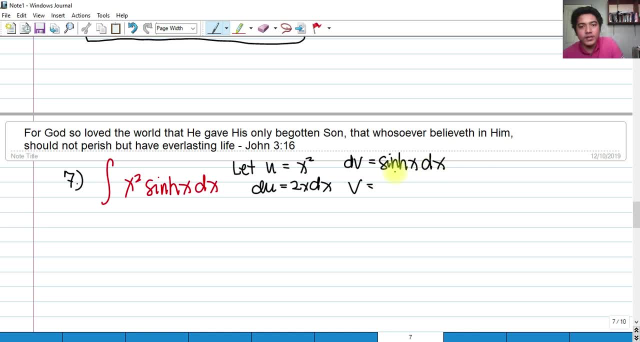 dx and if we're going to integrate this, this would be hyperbolic cosine of x. okay, and applying the formula we have, okay, we have uv, our uv is x squared hyperbolic cosine of x- okay, minus the integral of v, hyperbolic cosine of x. du is our 2x dx here, okay, and if i'm going to further solve this, what will? 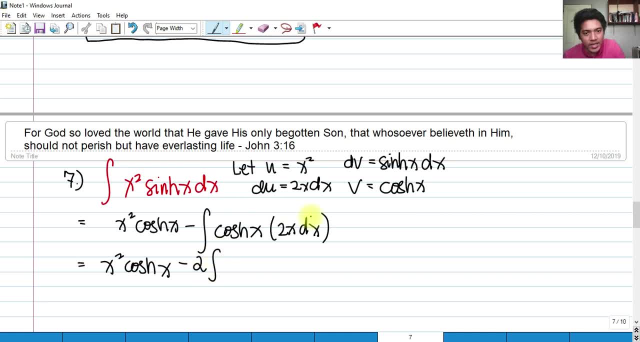 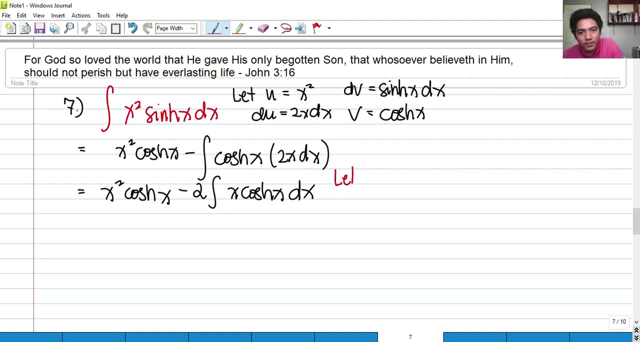 happen. i can factor out 2 outside of the integral sine, because that is a multiplication. so i have x, hyperbolic of cosine, of x, dx here, okay, and this is again an integral yielding to another integral. so we have to let another ibp, i mean we have to let: u is equal to x, du is equal to dx, our dv again is hyperbolic. 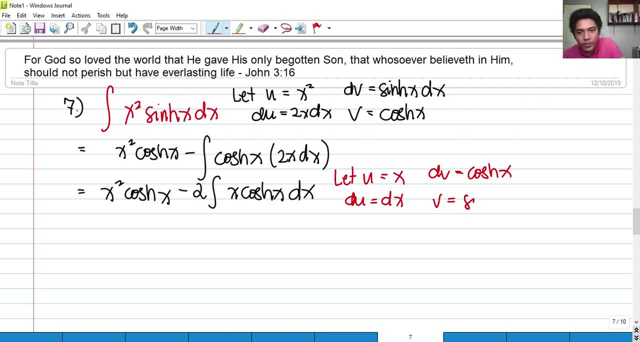 cosine of x and our v is hyperbolic sine of x. okay, so what will happen? apply again the formula: we have x squared, hyperbolic cosine of x minus 2. okay uv. we have u x hyperbolic sine of x minus the integral of v. du- hyperbolic sine of x. our dv is equal to dx. okay, so we have x squared. 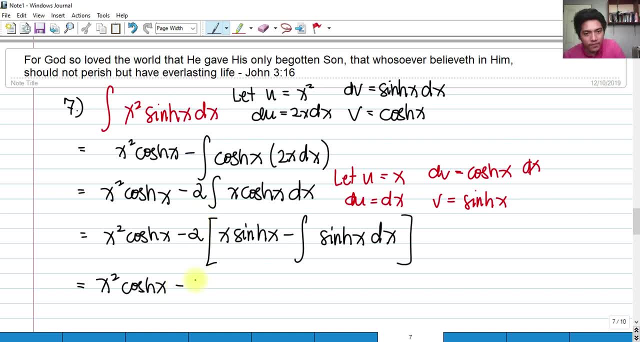 hyperbolic cosine of x distribute. we have negative 2x hyperbolic sine of x distribute. so the the integral of the hyperbolic sine of x is simply hyperbolic cosine of x. i've been going to distribute this negative 2 with the negative, that would be positive 2 and the integral of this. 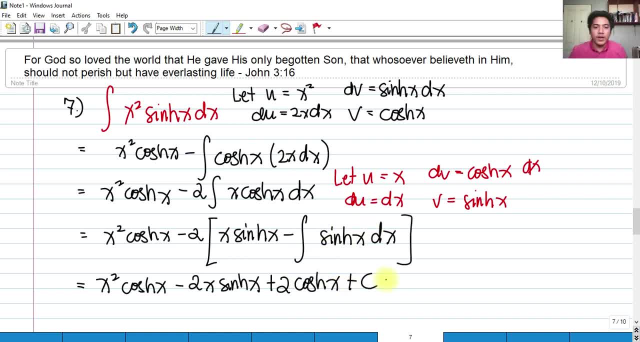 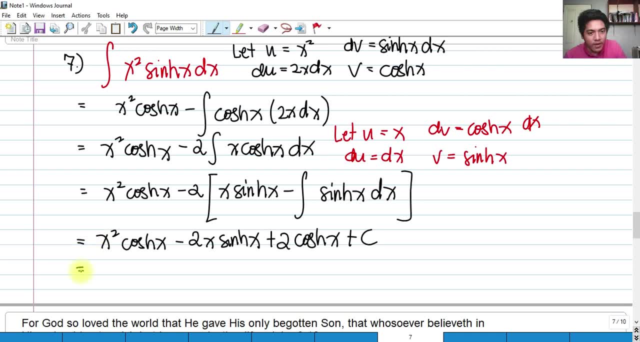 is hyperbolic cosine of x. don't forget the plus c, of course. and as you can see here, we can factor out cosine or hyperbolic cosine of x by: we have hyperbolic cosine, oops, we have hyperbolic cosine of x. is e multiplied by x squared plus 2? okay, this is that term and this term minus 2x, hyperbolic.